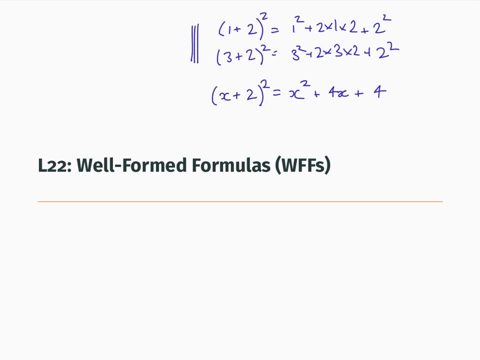 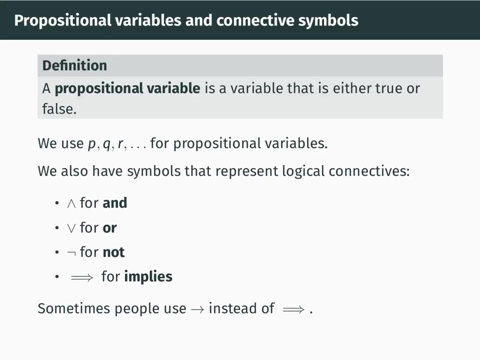 We're going to develop a formal language for expressing propositions and the variables that we use will be called propositional variables and instead of the x here which could have been a real or a complex number our proposition variables will be able to be true or false and instead of formulas like this one or expressions like like this one the formulas we will introduce in logic will be called well-formed formulas so those are the subject of this video so in our formal language we need first of all to have variables and the kind of variables we will use will be called propositional variables and here's the definition of a propositional variable propositional variable is a variable which can take the value either true or false if you happen to have done any computer programming before then this is like the concept of a bool or a Boolean variable traditionally we use symbols like P Q R S and so on for propositional variables so as I say we're going to develop a formal language for representing propositional that for representing propositional variables we're going to develop a formal language for 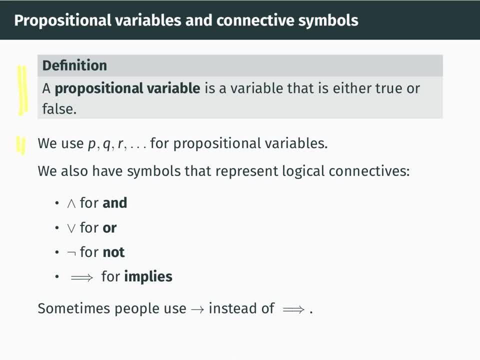 representing propositional that for representing propositional variables and in that language we need our variables are propositional variables will also need some brackets but the really important thing is we also need logical connectives so we have symbols that represent the logical connectives which we discussed in the previous video here are the symbols that we're going to use we're going to use first of all this wedge symbol for the connective and we're going to use this V symbol for the connective and we're going to use this V symbol for the connective and or we're going to use this symbol for not and this double arrow for implies now this implies symbol especially is not universal you'll often see people using a single arrow instead of implies and also you will sometimes see people just using the words and or not or implies instead of these symbols especially when you do some of your online quizzes you might have to type and or or or not instead of using these symbols mainly the reason I've set the quizzes up to do that is because it's rather difficult to type these special symbols whereas it's very easy to type words like and or not okay so let's 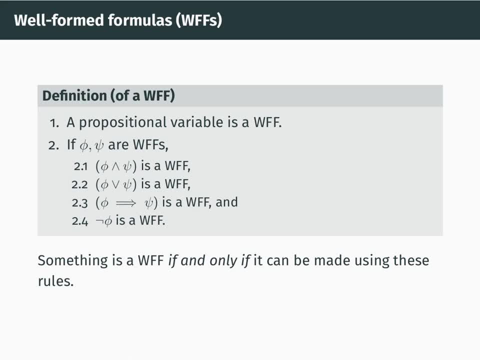 think a little bit about about the what we're trying to do here which is to develop a formal language for expressing propositions you're going to need to have a formal language for expressing propositions this is a bit like natural languages like English I mean in English you have a bunch of letters A B C and so on and some combinations of those letters make legitimate words you can see lots of examples of that on this slide but some composite some combinations of letters don't make legitimate words like if somebody writes X V E N T U I L D that's all of the things which make that up our legitimate English letters but it doesn't make a meaningful English word so we need to distinguish between the sequences of logical symbols and propositional variables and brackets which do make meaningful logical expressions and meaningful propositions and ones which don't and for us meaningful well-formed expressions will be called well-formed formulas and on this slide we're going to give a definition of a well-formed formula and formula, but it's quite an unusual definition. It's a type of definition you're perhaps not 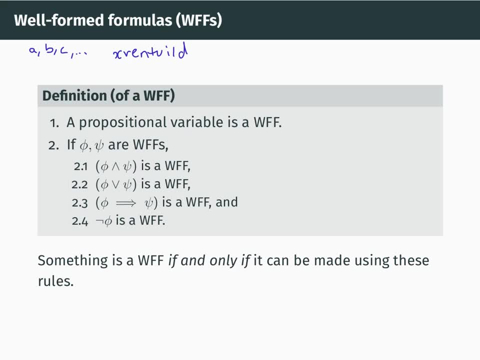 familiar with called a recursive or an inductive definition. So here's the definition of a well 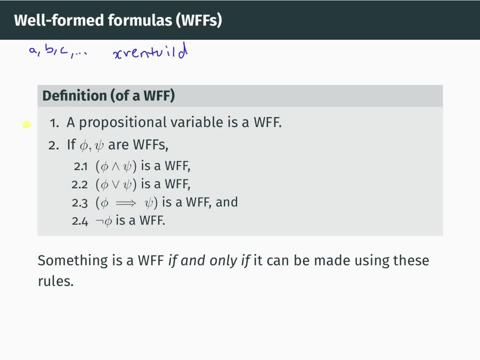 formed formula. It comes in two parts. And the first part is that any propositional variable on its own is a well formed formula, WFF for short. The second part of the definition is split into four parts. And what it says is that if you have two well formed formulas, phi and psi, then firstly, phi and symbol psi in brackets is a well formed formula. Secondly, phi or symbol psi in brackets is a well formed formula. Thirdly, phi implies symbol psi in brackets is a well formed formula. And finally, the not symbol followed by phi is a well formed formula. So let me stress that this definition completely describes what is and is not a well formed formula. Something is a well formed formula if and only if you can make it using these rules. 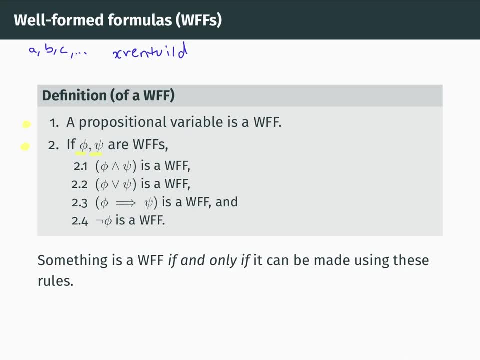 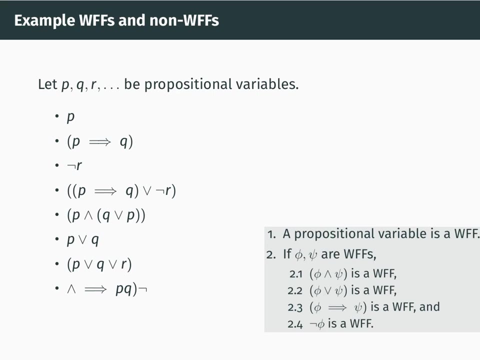 Let's now look at some examples of well formed formulas and things which are not well formed formulas. So I've copied at the bottom of the screen here this definition on the previous slide of what is a well-formed formula it's something which can be built using our two rules so on this slide we will take P and Q and R as usual to be propositional variables and we're going to look at some examples of things which are well-formed formulas and things which are not well-formed formulas so our first example here is just the propositional variable P and that is a well formed formula green tick it is a well-formed formula by rule 1 Rule 1 says that every propositional variable on its own is a well formed formula said this P on its own is a well formed formula next example here so P implies symbol Q in brackets it is a pre- well-formed formula and the reason is that P is a well-formed formula by rule one Q is a well-formed formula formula by rule 1. And then rule 2.3 here says that if you have two well-formed 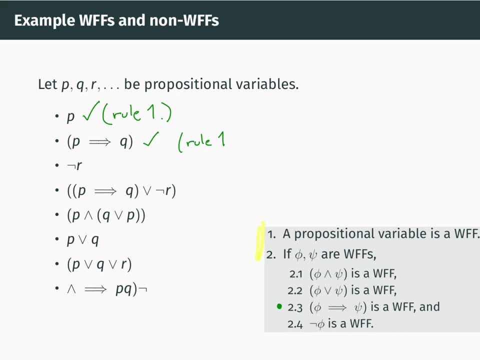 formulas, phi and psi, then phi implies psi in brackets is a well-formed formula. So using rule 1 and rule 2.3 I get that P implies Q in brackets is a well-formed formula. Next example, not R, again this is a well-formed formula and the reason that this is a well-formed formula is that first of all by rule 1, R on its own is a well-formed formula and next by rule 2.4, if you've got a well-formed formula phi and you stick a not symbol in front of it then the result is again a well-formed formula. 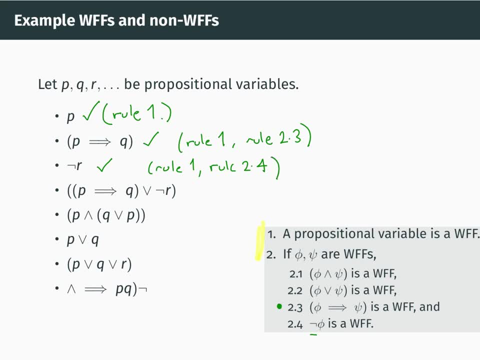 so not r is a well-formed formula next example more complicated example again this is a well-formed formula and again the reason it's a well-formed formula is because you can make it using our sets of rules for making well-formed formulas so we already know that brackets p implies q brackets is a well-formed formula that was our second example and now so what was that that worked by rule one and then rule 2.3 now we can apply rule 2.2 to say that not r is a well-formed formula that was our example here 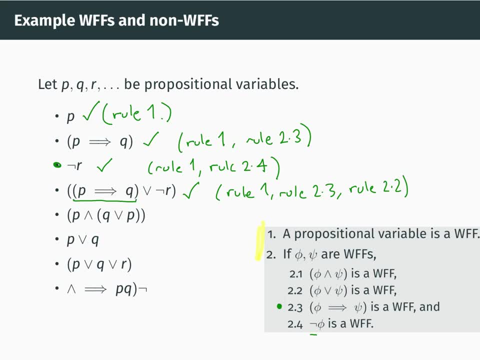 p implies q and brackets is a well-formed formula that was our example two 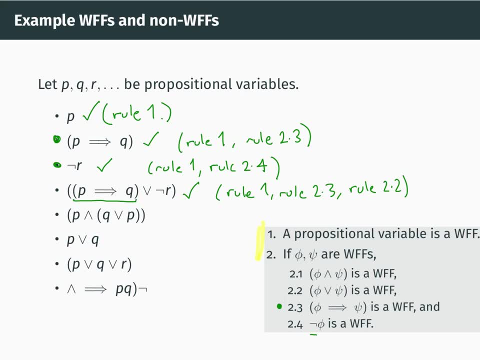 and so by rule 2.2 this whole thing is a well-formed formula okay again similarly i'm not going to write out the full justification this time but again this next one is a well-formed formula and this time the reason is that you can use first of all rule 2.2 to get that brackets q or p is a well-formed formula and then you can use rule 2.1 to get that brackets p and q or p is a well-formed formula 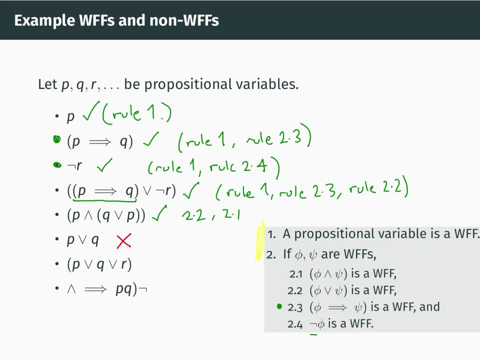 okay next however this thing is not a well-formed formula it's nearly a well-formed formula but it's missing brackets so let me stress once more if you want a well-formed formula you must follow these rules and there is no set of rules which allow you to make this as a well-formed formula you can use 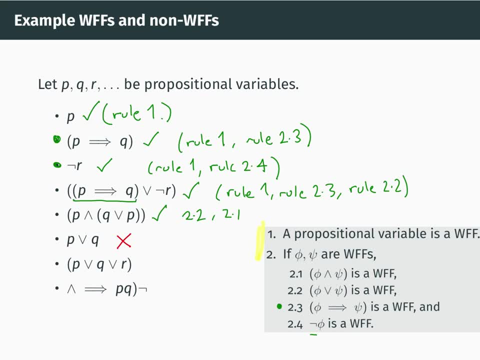 if you like rule one that says p and q on their own well-formed formulas and then you you can use rule 2.1 to get that brackets, excuse me, rule 2.2 to get that brackets P or Q is a well-formed formula. But without the brackets, that is not a WFF. 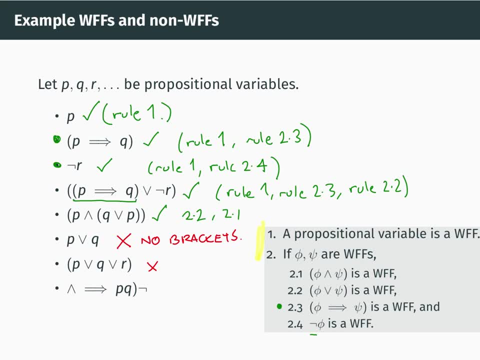 Again, the next example is not a well-formed formula. There is no well-formed formula rule which allows you to produce this. Again, it's really close to being a well-formed formula. 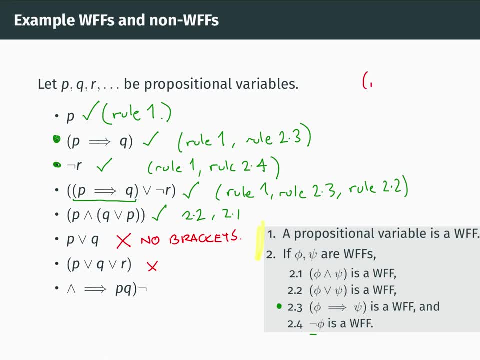 If you had just another set of brackets, like if you had something like P or Q or R, that thing would be a well-formed formula. But there is no way of using the rules here